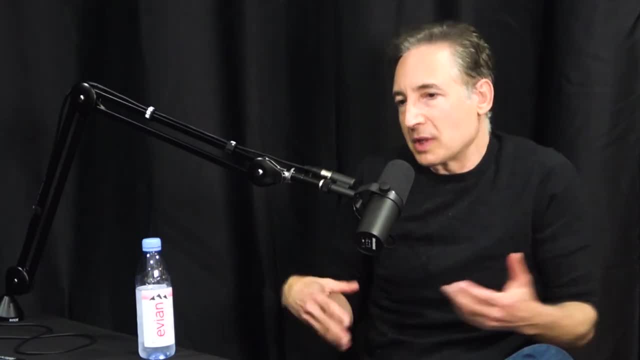 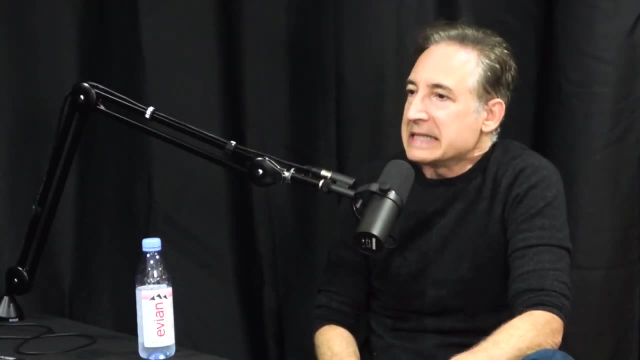 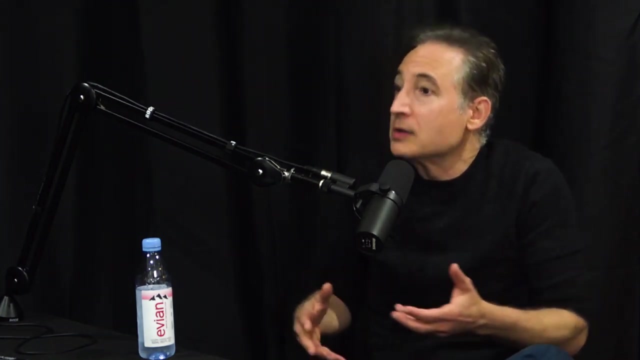 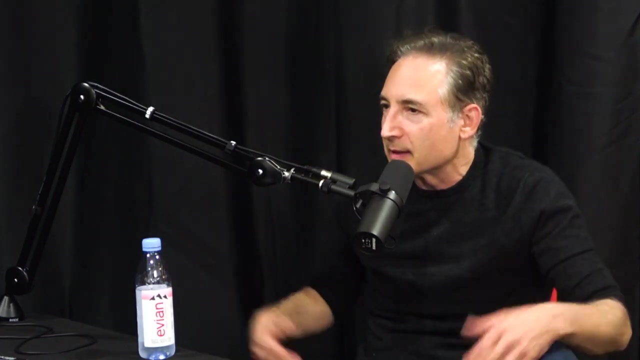 Biology is just small details, we'll figure out. Yeah, So it is really trying to put gravity and quantum mechanics together, And since I was a college kid, I was deeply fascinated with gravity And, as I learned, quantum mechanics, the notion of physicists being stumped and trying to blend them together. how could one not get fired up about maybe contributing something to that journey? 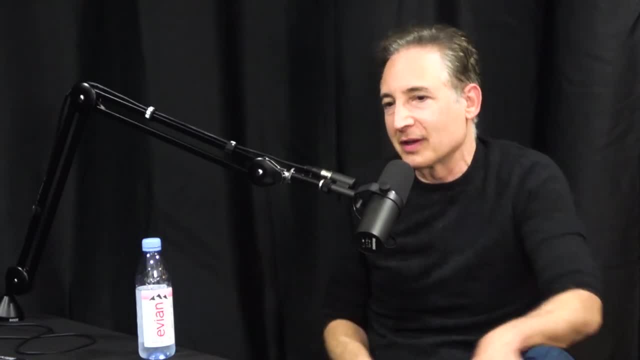 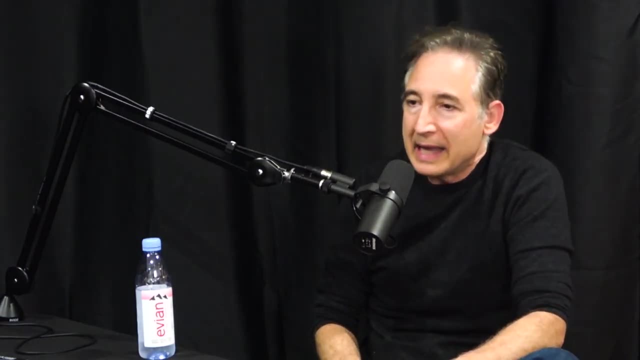 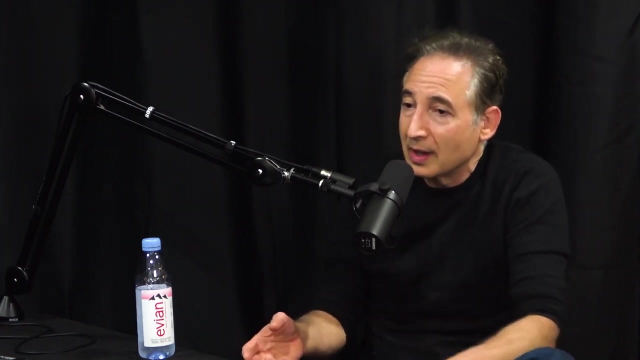 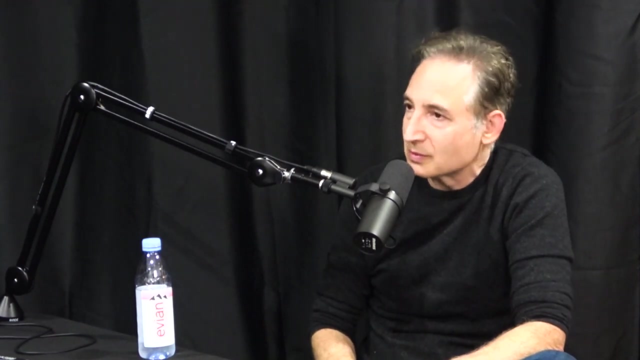 And so we've been on this. you know, I've been on this for 30 years, since I was a student. We have made progress. We do have ideas. You mentioned string theory is one possible scenario. It's not stuck. String theory is a vibrant field of research that is making incredible progress, but we've not made progress on this issue of experimental verification, validation, which is, you know, it is- a vital part of the story. 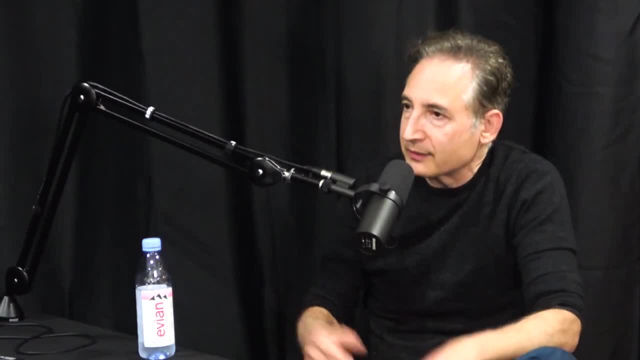 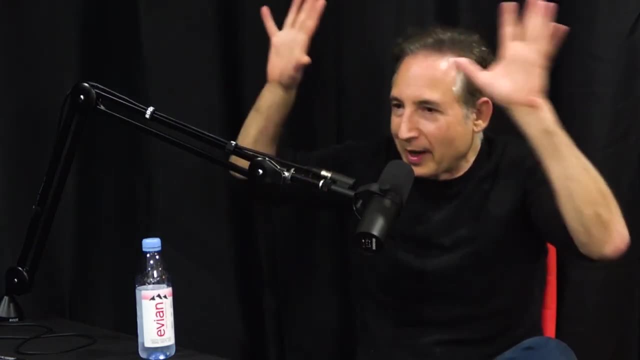 So I would have hoped that by now We would have made contact with observation If you would have interviewed me back in the 80s when I was, you know, a wild, bright eyed kid trying to make headway, working 18 hours a day and this sort of stuff. 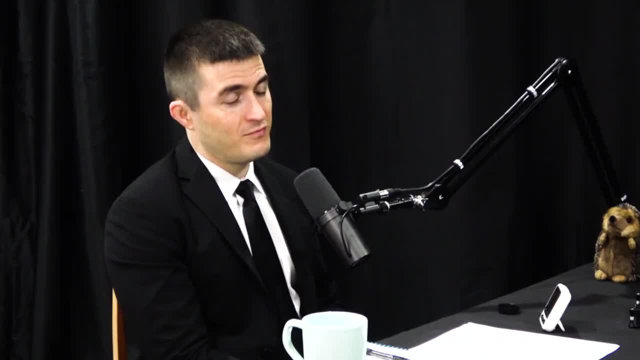 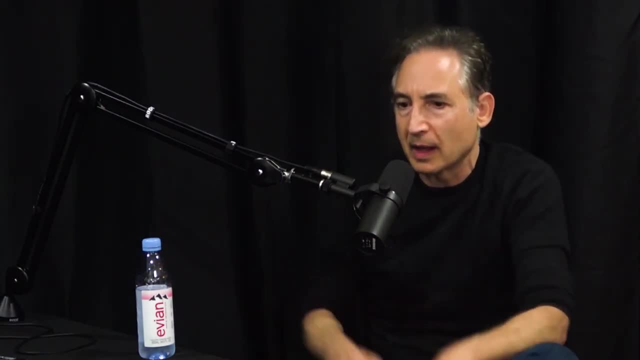 I would have said, yeah, by by 2021.. Yeah, we're going to know whether it's right or wrong, We'll make contact. I would have said, look, there may be certain mathematical puzzles that we've got to work out, but we'll know enough to make contact with experiment that has not happened. 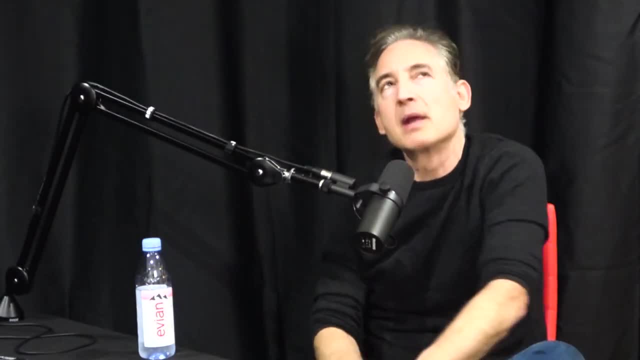 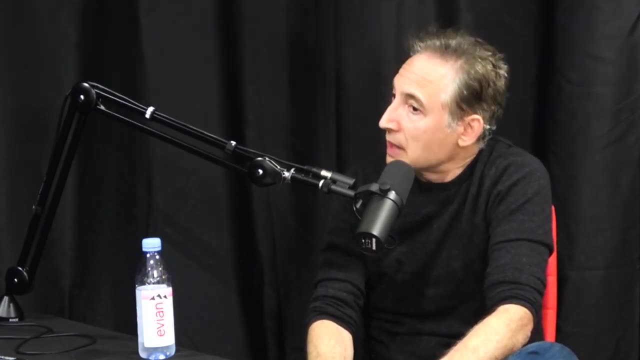 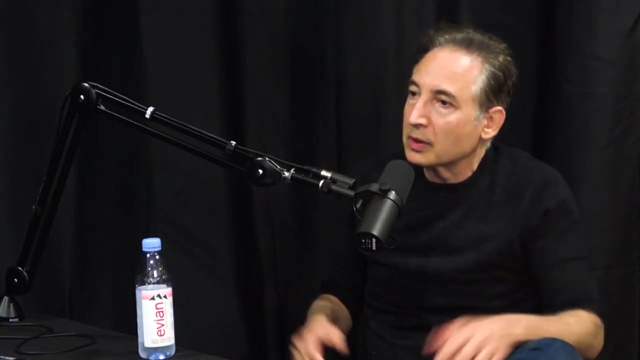 On the other hand, if you would have interviewed me back then and asked me: will We be able to talk about detail, qualities of black holes and understand them at the the level of detail that we actually, I would have said no, I don't think that we're going to be able to do that. 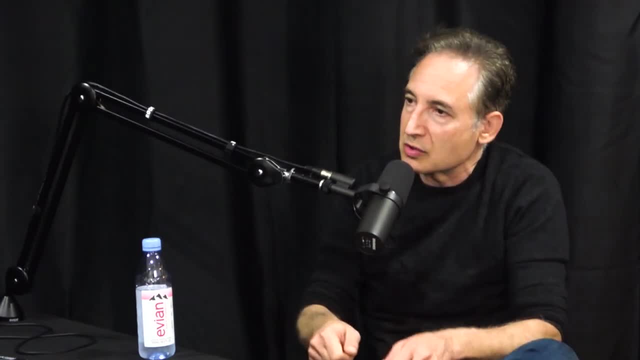 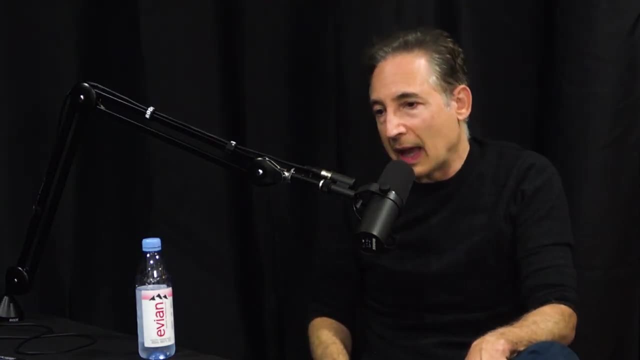 Will we have a, an exact formulation of string theory in certain circumstances? No, I don't think we're going to have that, And yet we do. So it's just to say you don't know where the progress is going to happen. But yes, I do hold out, hope that maybe before I move on. 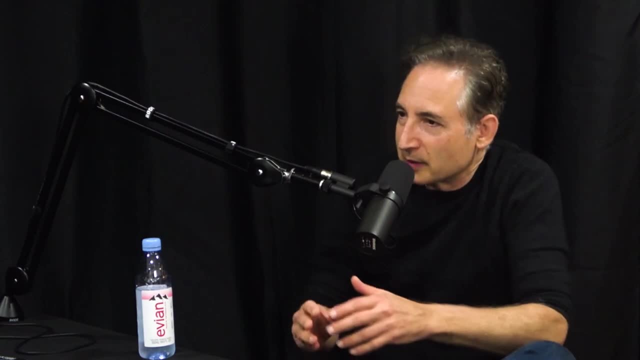 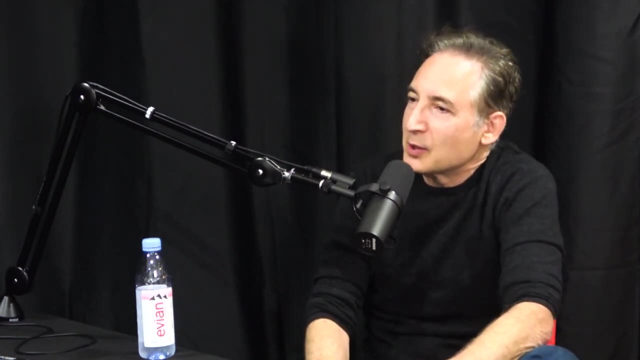 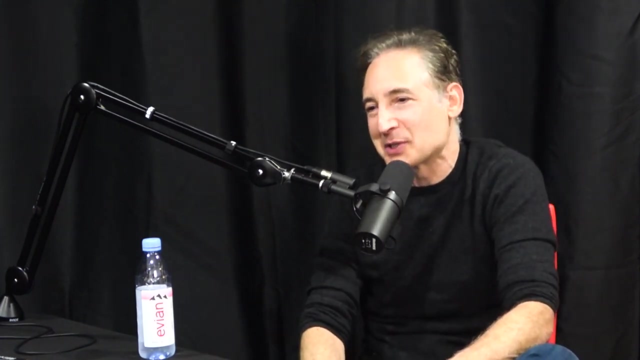 To wherever? I don't think there is an after, but I would love, before I leave this earth, to to know the answer. But you know science and the universe. it's not about pleasing any individual. It is what it is, And so we just press onward and we'll see where it goes. Thank you very much for your time.